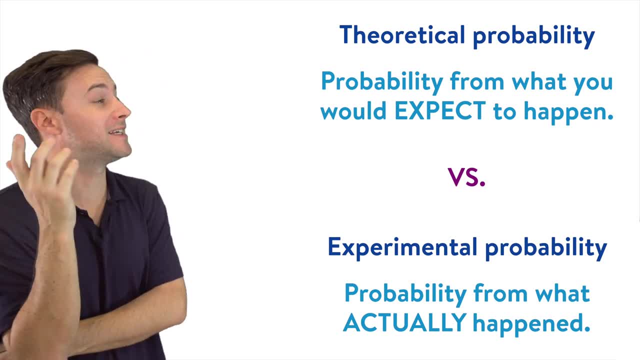 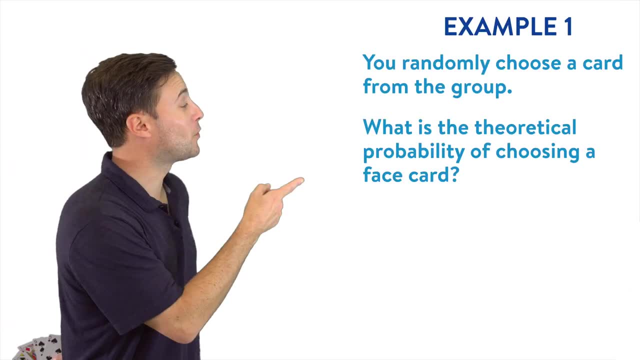 to happen, whereas an experimental probability is based on what actually happened in your experiment. All right, hopefully all that makes sense. Let's move on to our first example. All right, example one: You randomly choose a card from the group. What is the theoretical probability? 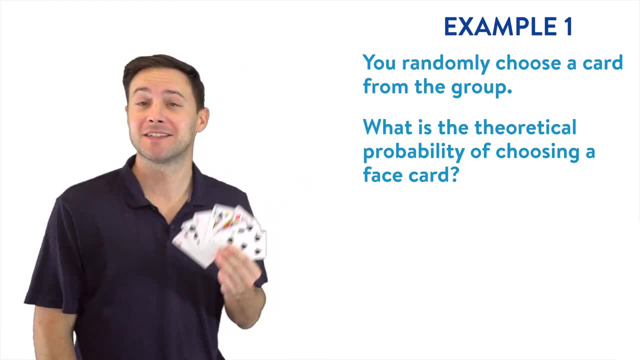 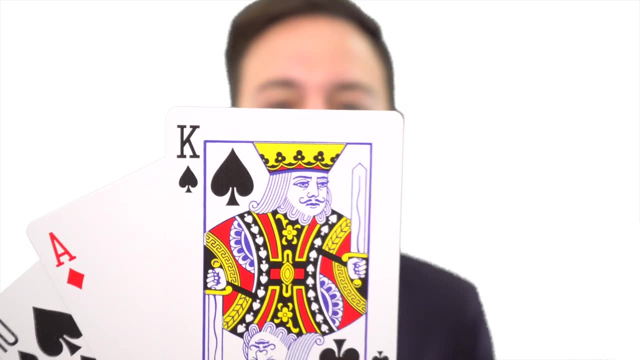 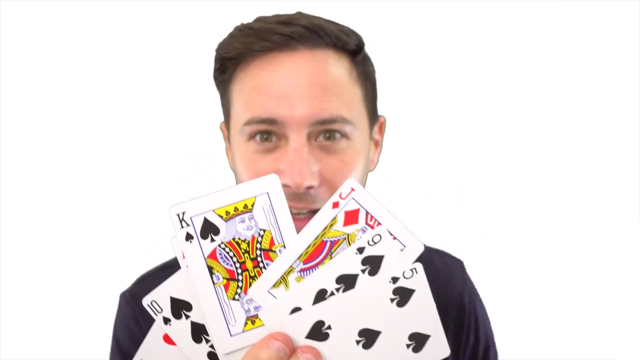 of choosing a face card. All right. well, first, what are face cards? A face card is a card that has a face on it, just like that. So if you look here, the face card is a face card that has a face on it and the face cards are the jack and the king. Okay, 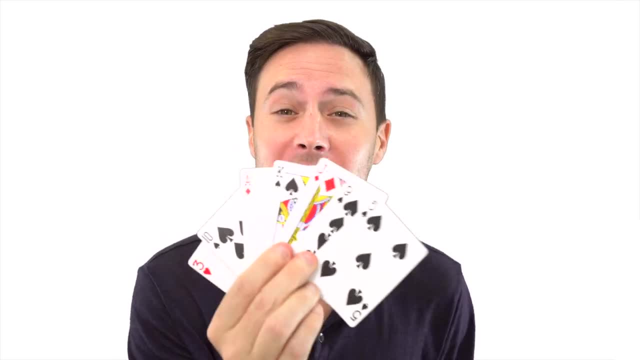 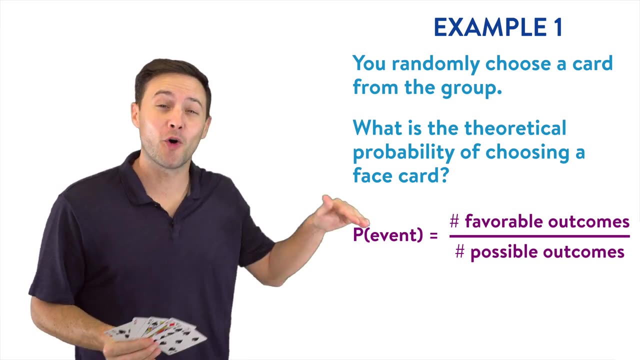 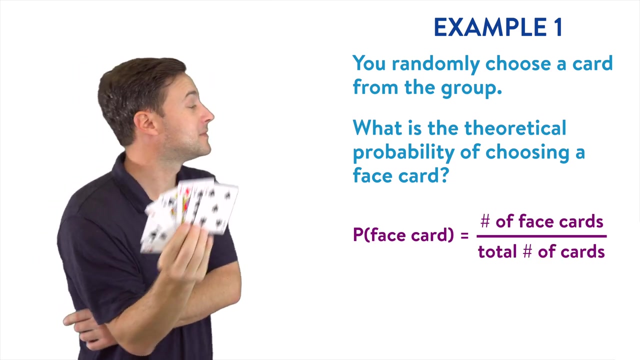 Queen would also be a face card, but there's no queen here. So with that now we can calculate the theoretical probability. So the probability of the event is the number of favorable outcomes over the number of possible outcomes. So for this one probability of a face card is going to be equal to 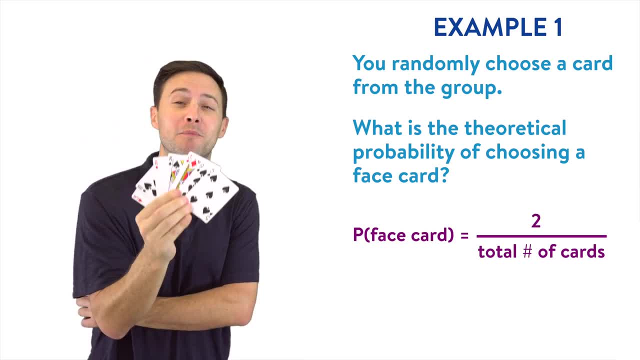 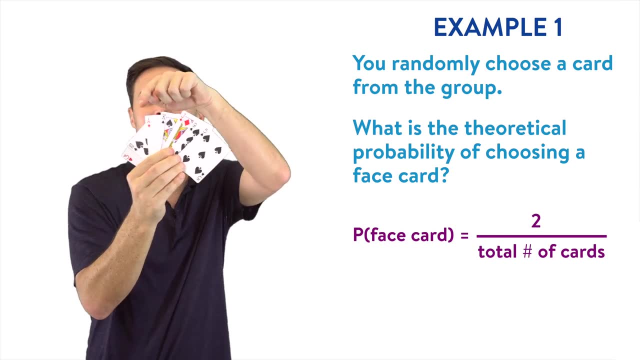 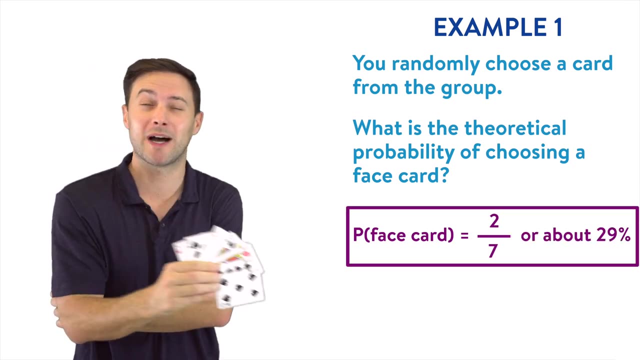 two divided by the total number of cards, because each card is a possible outcome. And how many cards are there? One, two, three, four, five, six, seven. So the theoretical probability of choosing a face card is two-sevenths or about 29%. Let's try another example. 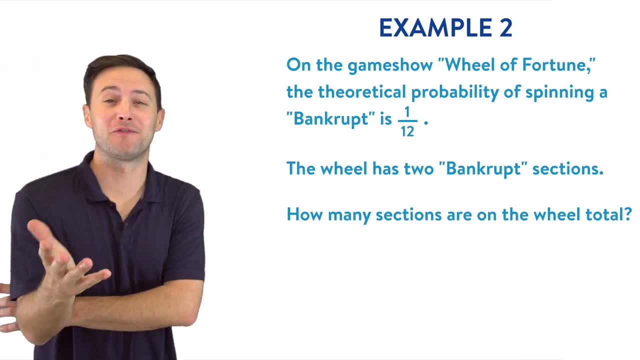 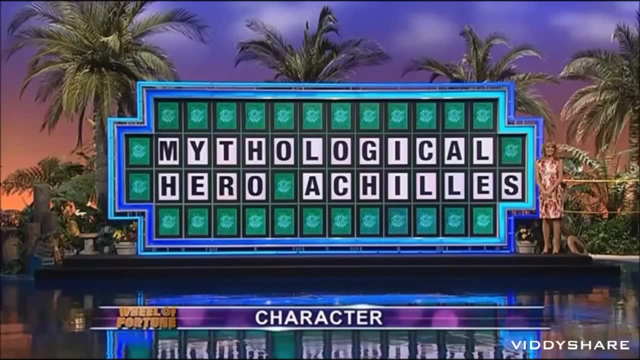 All right. example two, On the popular game show Wheel of Fortune. Okay, nice, solve, That would be a good idea. yeah, Mythological hero Achilles, You can't accept that. Okay, Shelby, I'll solve Yeah. 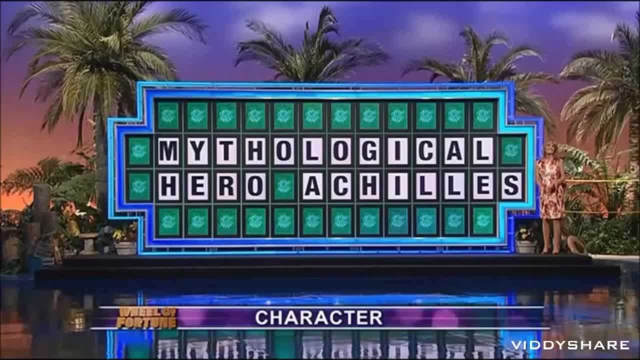 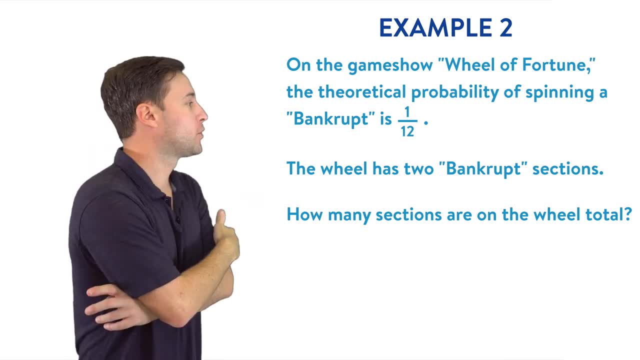 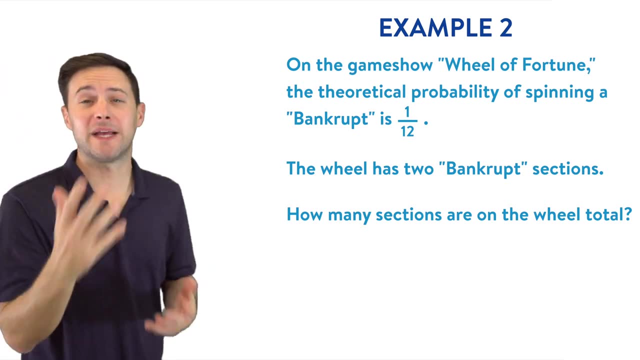 Mythological hero Achilles. Yeah, that's it. The theoretical probability of spinning a bankrupt is one-twelfth If the wheel has two bankrupt sections. how many total sections are on the wheel? All right, so on this question, basically, they're giving us a theoretical probability. 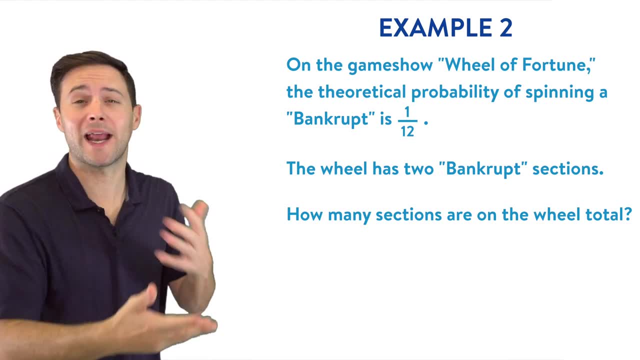 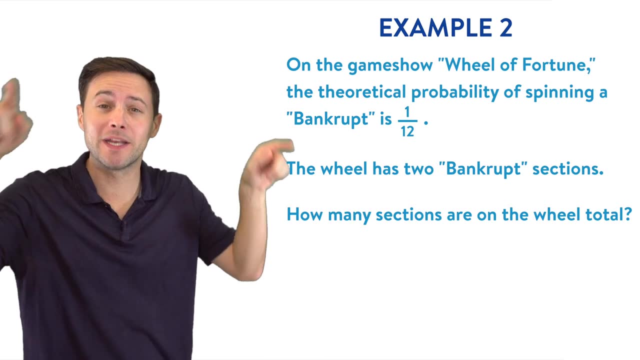 and we're going to use that not to make a prediction- and that's a prediction of what might happen in the future- But we're going to use it to help find missing information, And in this case, the missing information is how many total sections are on the wheel. 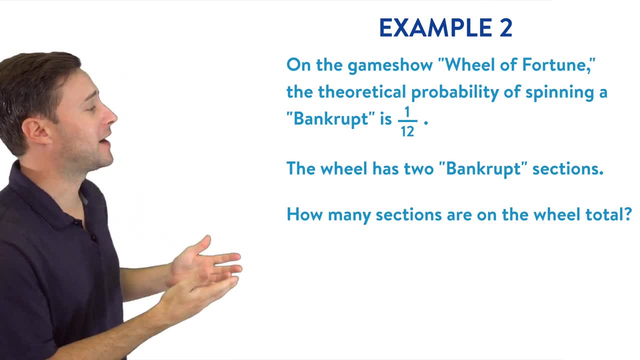 So to do this multiple different ways on how you can find that out, We could do a ratio table, we can do some algebra, but I'm just going to set up a proportion. So our theoretical probability of going bankrupt is one-twelfth. 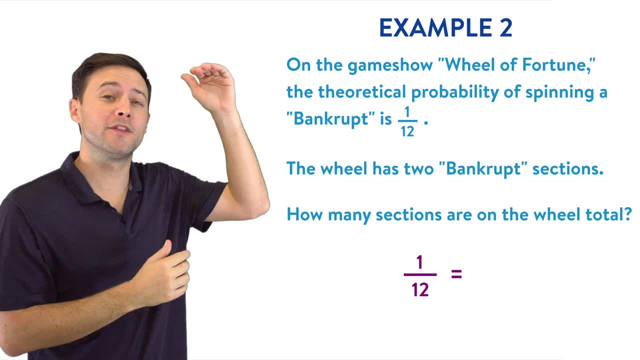 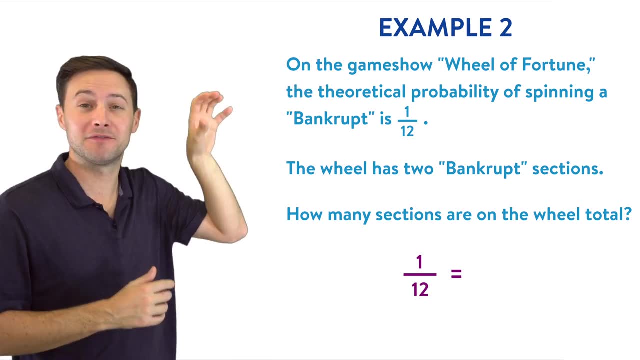 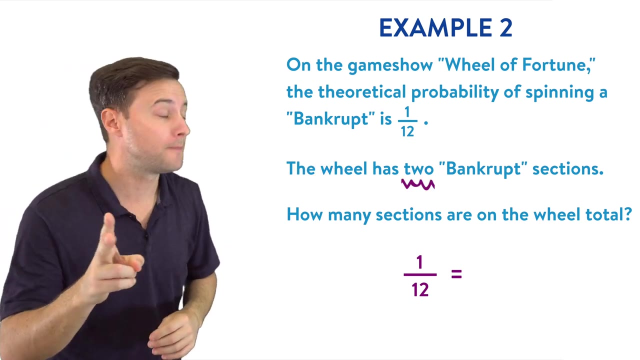 That's going to be equal to well that one in the next row, the numerator that represents the favorable outcomes. So one bankrupt out of 12 sections is what. that would basically mean 12 total outcomes, But we know that there's actually two bankrupt sections, So 1: 12 is going to be equal to there's 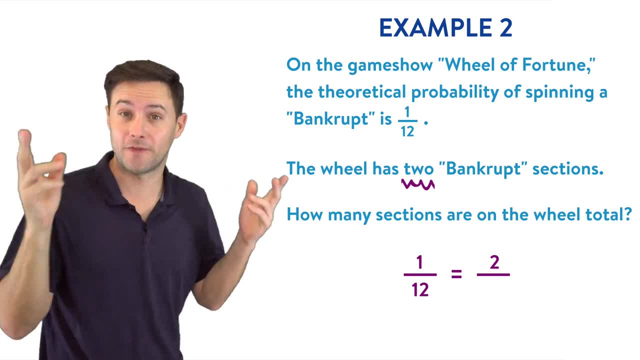 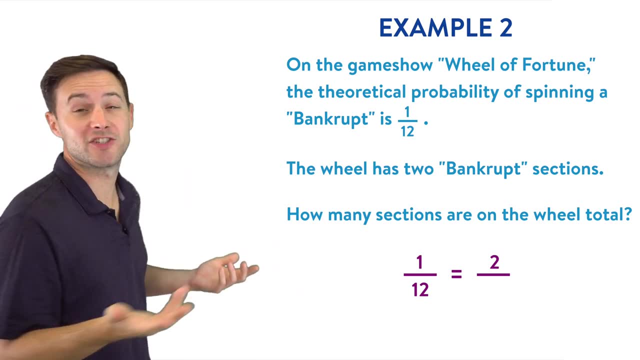 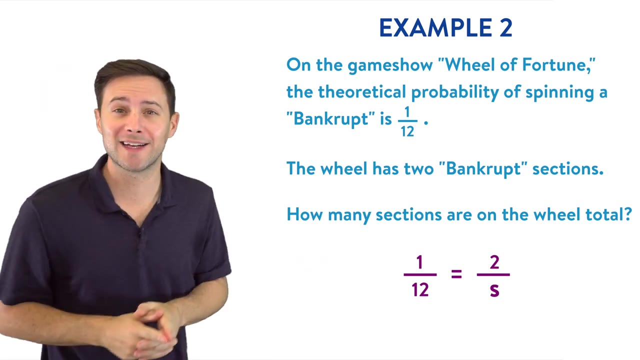 two bankrupt sections. So that goes in the numerator, our favorable outcomes divided by the total number of outcomes, which is what we're trying to find. Let's just call that S for sections. So 1- 12 is equal to 2 over S. This one's pretty. 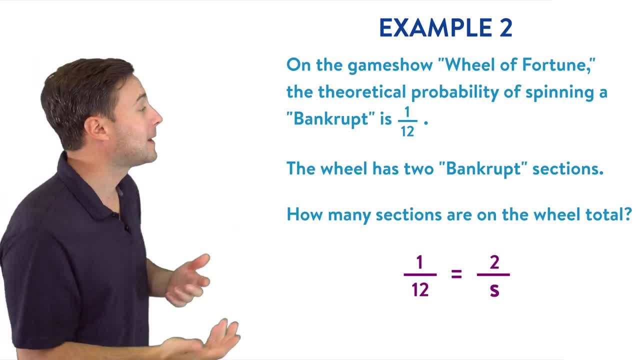 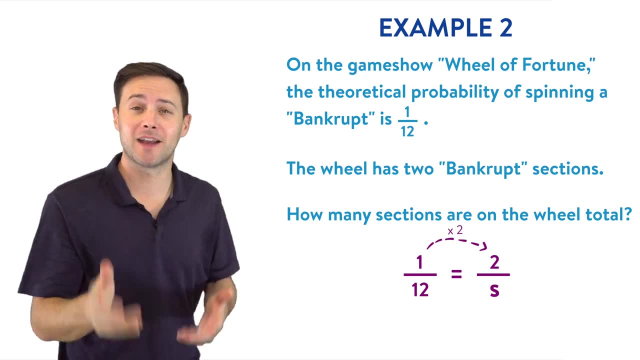 simple Again. you could do some algebra if you want, but I'm just going to use some mental math. To get from 1 to 2, we just multiply by 2.. So if I do the same to the denominator, 12 times 2 will give me 24 total sections on the Wheel of. 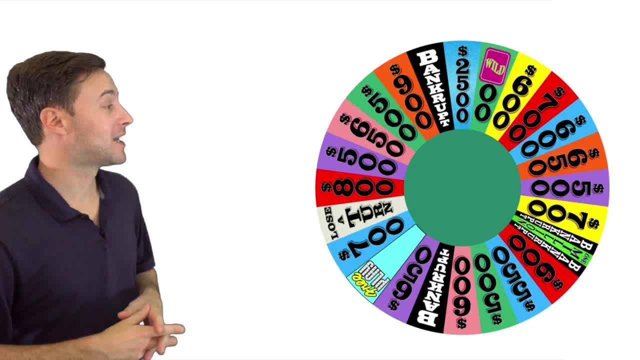 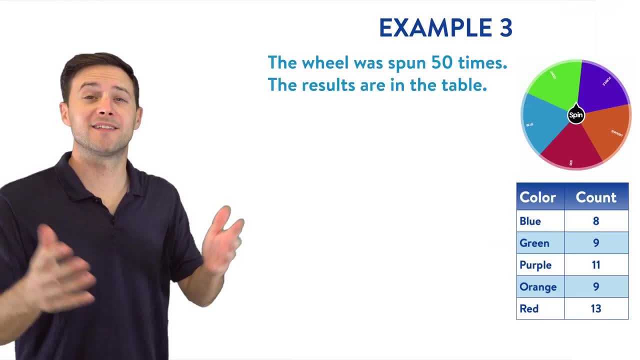 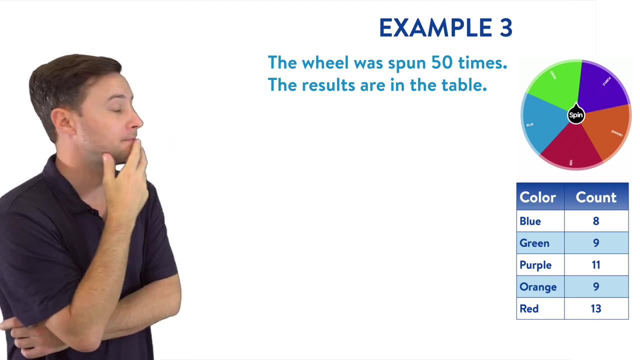 Fortune, Which is true, by the way. if you want to double-check me, Alright. here's something to remember To try on your own, Alright. here's our last example. You spin the spinner 50 times and the table shows you all the results of those 50 spins. So Part A says what is. 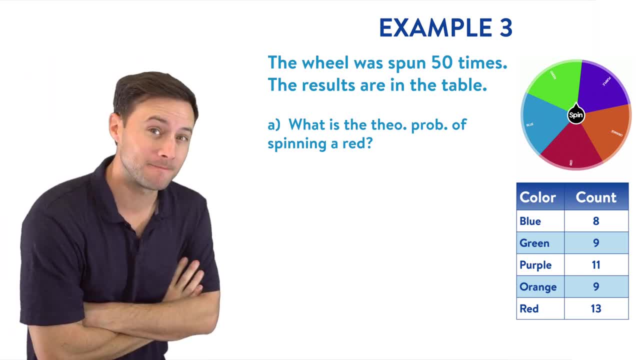 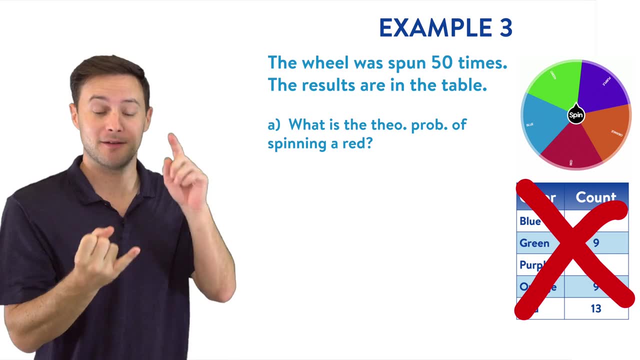 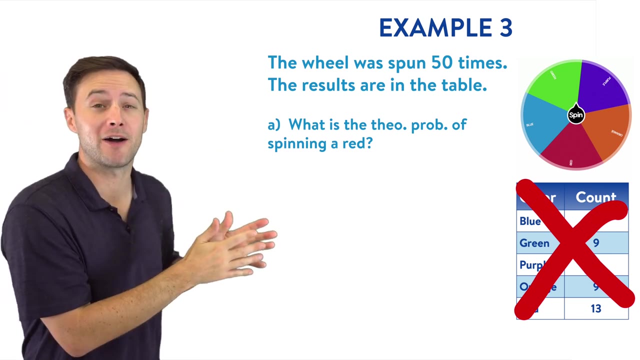 the theoretical probability of spinning a red. Well, for theoretical probability we don't need to even look at those results. We just need to look at how many favorable outcomes are there and what are the total possible outcomes. So the favorable outcomes would be red and there's only one red. 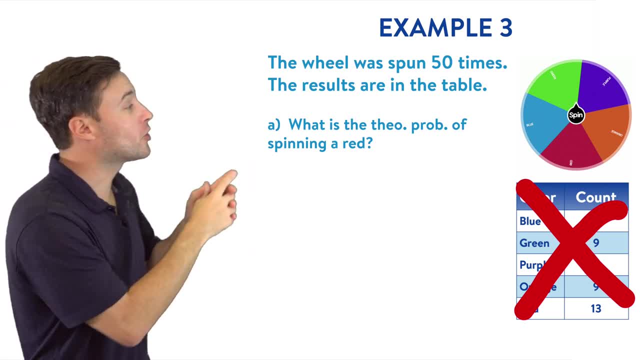 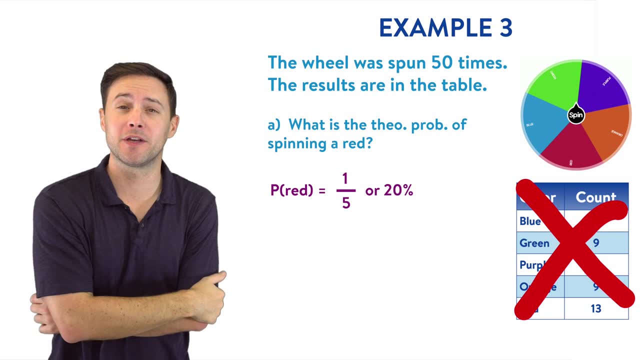 section. So that's 1,. pretty simple. And then the total outcomes. well, how many sections are on the spinner? And that's 5.. So our theoretical probability of spinning a red is one-fifth or 20%. Pretty simple. 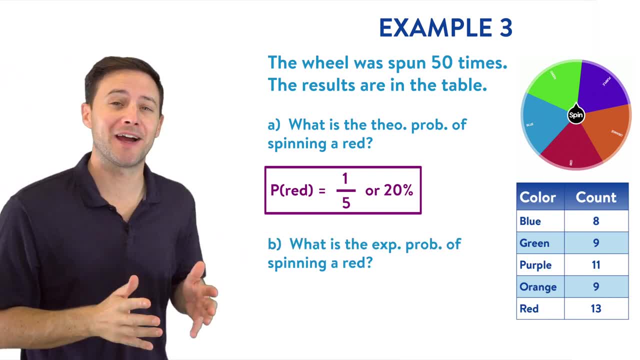 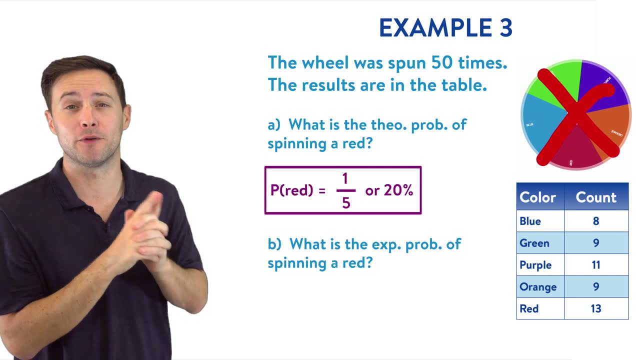 Let's move on to Part B. So Part B: now we need to find the experimental probability of spinning a red. So Part B: now we need to find the experimental probability of spinning a red, And for that we do need to look at the table and the results. 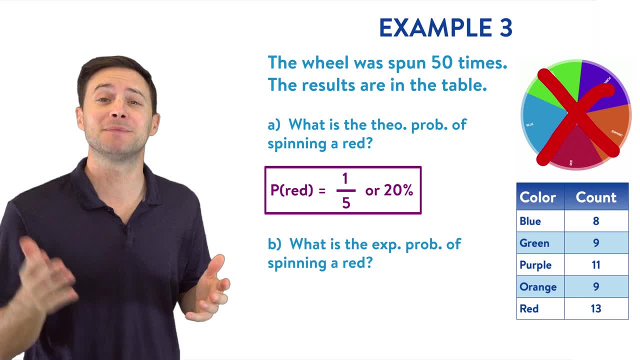 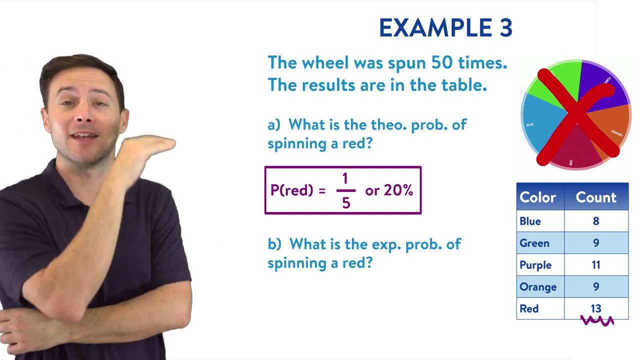 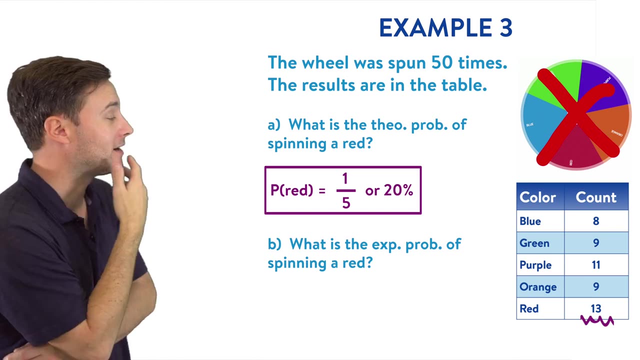 So for the experimental probability, how many times did the spinner land on red? And if we look at the table, it was 13 times And then so that goes in the numerator And in the denominator. how many times did we do the experiment? Did we spin the spinner And 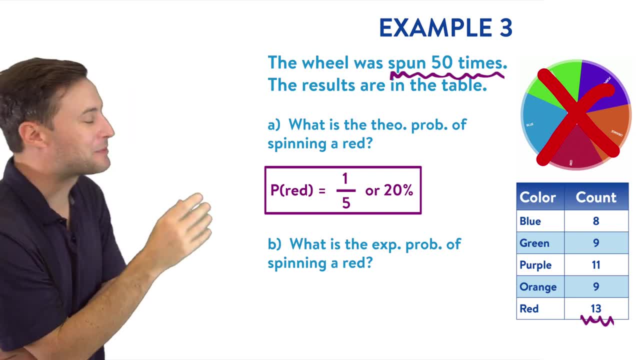 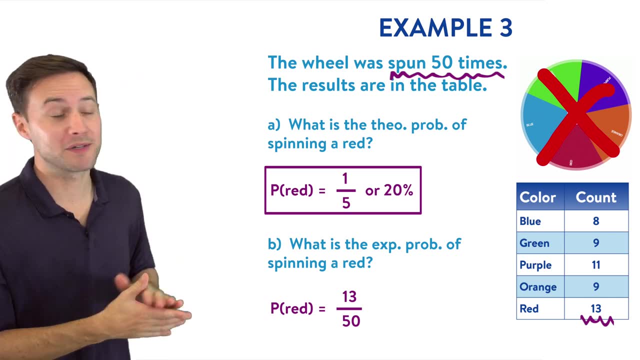 if you remember, it was 50 times. So the experimental probability of spinning a red is 13 times. So if you think about all of that, that minus 15 to the potential probability of spinning a red is 26 times. If you think about all of that, that is lower than 72.. But that is just minus 22, which 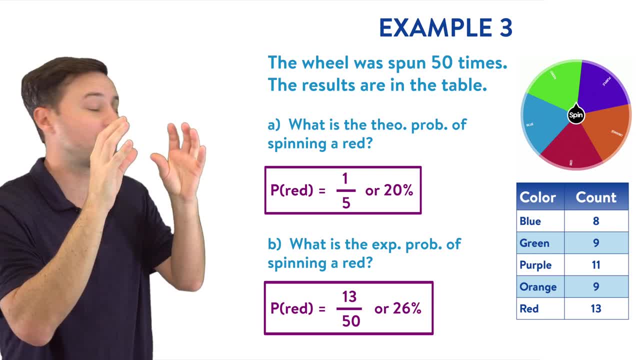 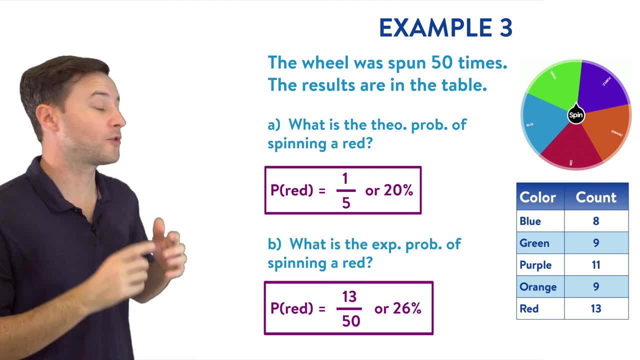 is 1st minus 7, which is 7.. So if you cannot put that in, it would cost you 1 free per minute amongst just 1, and that would be about a hundred million dollars. So if you grow into a company, and this year if you're really focused on doing all sorts, 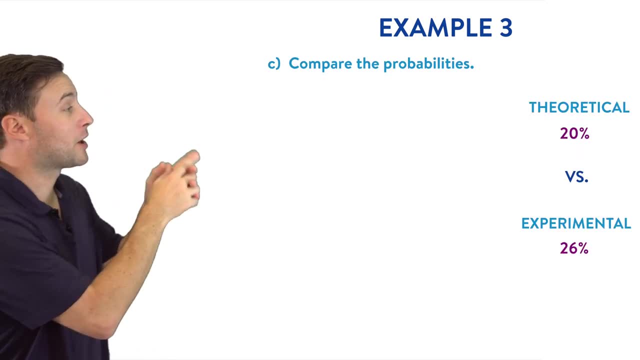 of stuff. you might be in a really good company, But we're together instead. So it's going to be 1, 1 Sagittarius against 1 is 23.. Alright, so all those things at 1, which is worth in the equation. So it all comes. 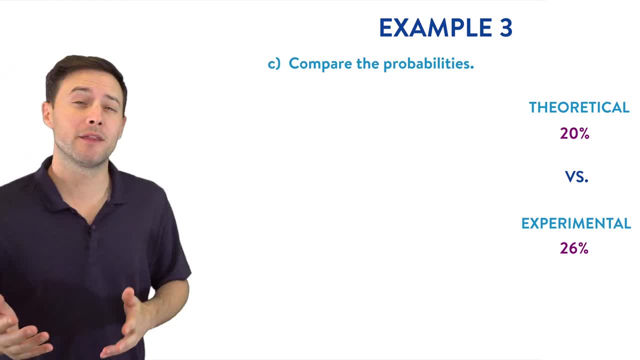 to 1, and let me just see that graph again. We're going to go take a look at that diagram. probability was greater than the theoretical probability and you might be thinking, well, why would that be the case? and you have to remember the theoretical. 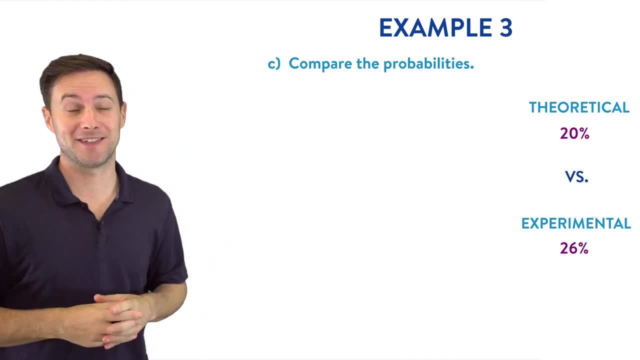 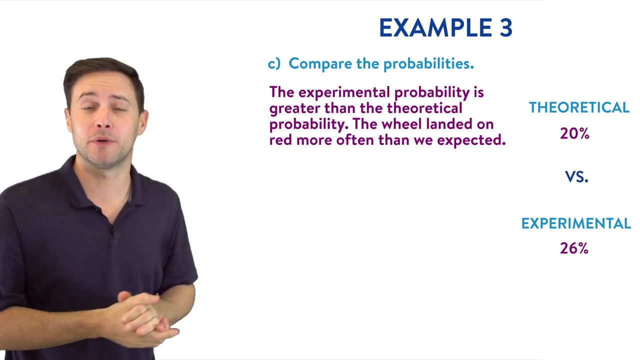 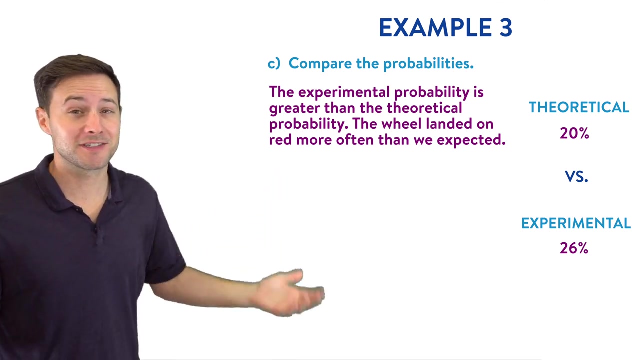 probability is theoretical. It's what you would expect to happen, but it's not what always happens. This is why casinos exist in the first place, or the lottery. So when we compare, we would say that the experimental probability is greater than the theoretical probability. and what might be a reason for that? Just luck. 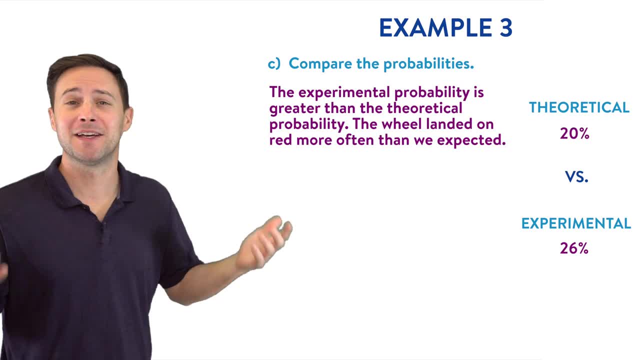 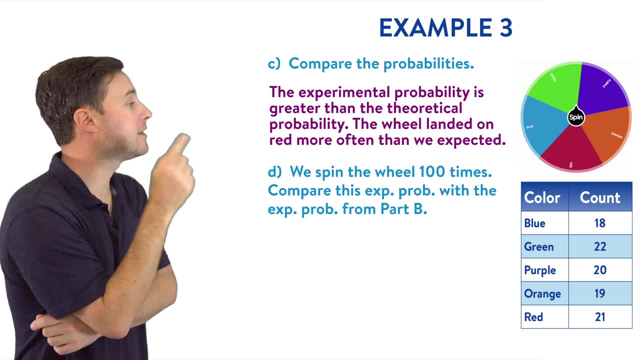 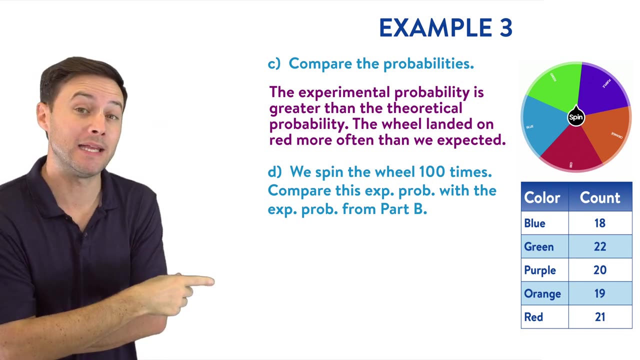 Just luck It happened to land on red more often than we expected. So part d says we spin the spinner 100 times. compare the experimental probability now at a hundred times compared to what we got in part b. So if you look at the